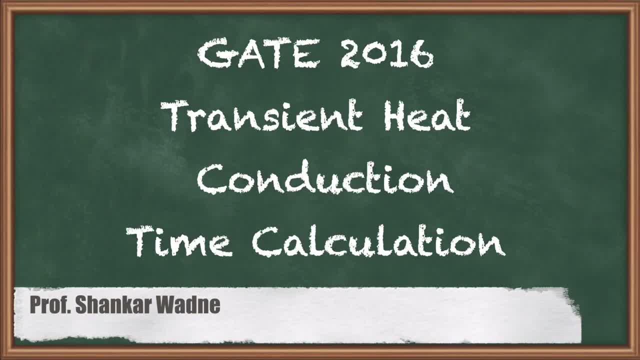 Hello, my dear students, in this lecture we are going to see one previous year gate numerical. This question was asked in gate 2016 for 2 marks in set 1.. This question was asked to find time required for the cooling, which is one of the questions, from transient heat conduction. 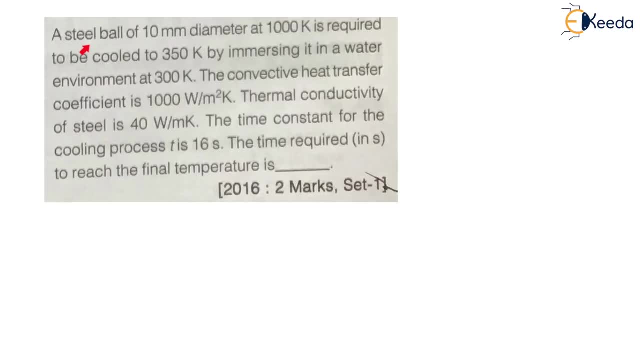 So let us understand the question. The question is a steel ball of 10 mm diameter. Now here they have given steel ball. The ball is always spherical. Therefore, let us draw this ball, Let us say this is a steel ball having spherical. 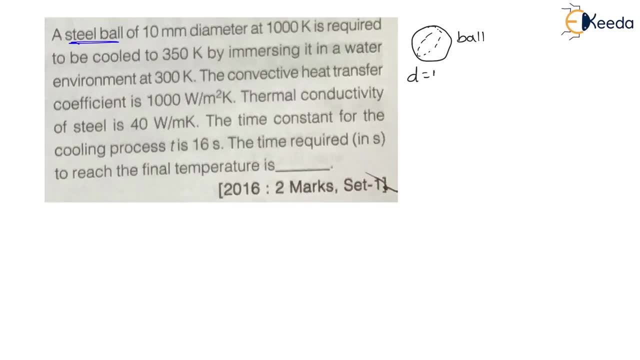 Now it is of. diameter is equal to diameter of ball is 10 mm, Which is also called as 10 into 10, to the power of minus 3 meter. Let us write down in meter A steel ball of 10 mm diameter at 1000 Kelvin. 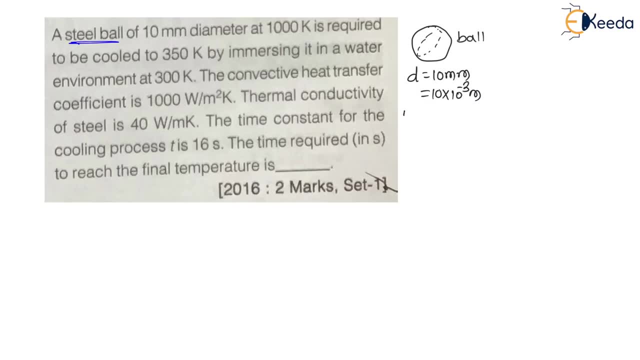 Now initial temperature of ball is 1000 Kelvin. Therefore here Ti is given 1000 Kelvin, Then is required to be cooled to 350 Kelvin. Now this ball we have to cool up to 350 Kelvin Means the temperature of ball we have to make 350 Kelvin. 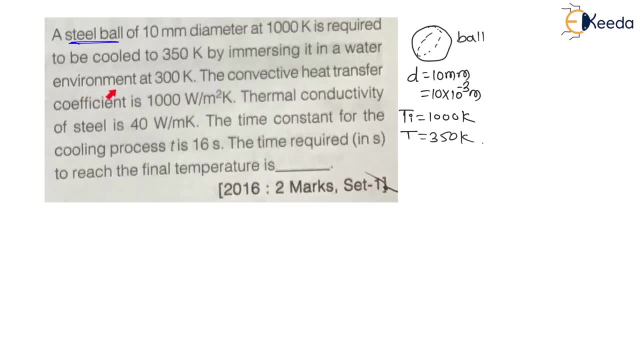 Right, By immersing it in the water environment at 300 Kelvin. Now the surrounding fluid is a water and the surrounding fluid temperature is 300 Kelvin. Therefore, we can say that T infinity surrounding fluid temperature is 300 Kelvin. Right, Then. the convective heat transfer coefficient is 1000 Watt per meter square Kelvin. 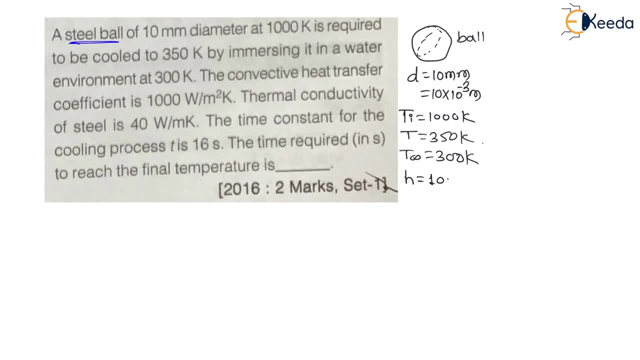 Therefore here they have given per water H value, That is, 1000 Watt per meter square Kelvin. Then the thermal conductivity of steel is 40 Watt per meter Kelvin. For this steel ball they have given thermal conductivity which is 40 Watt per meter Kelvin. 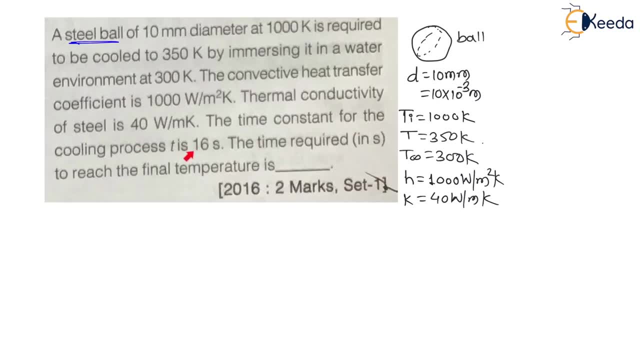 Right, Then the time constant for the cooling process T is 16 seconds. Now, this is not time, My dear students. this is not time. This is a time constant. Time constant is given Here. I will tell you what is time constant. 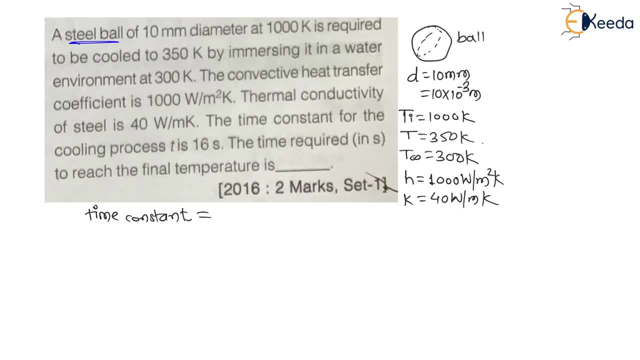 Time constant, which is nothing but 16 seconds. 16 seconds, It is not time. The question is to find time. Let us understand the question. The question is: the time required in second to reach the final temperature is Now from 1000 Kelvin to 350 Kelvin. 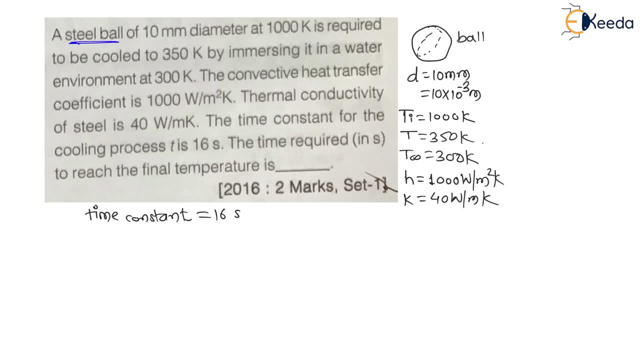 To reach this temperature. What is the time required? Right? So here time, small t in seconds. we have to find Right, And time constant is given. Now, my dear students, Let us assume lumped heat capacity analysis. That is, lumped heat capacity analysis is nothing but transient heat conduction. 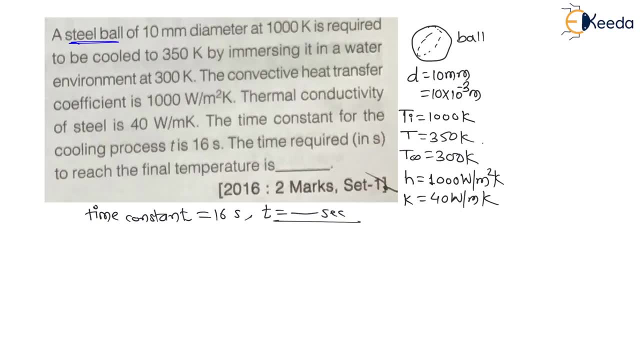 And my dear students for this transient heat conduction We have derived the formula That is. the formula is final temperature T minus fluid temperature T infinity. They have an initial temperature Ti minus fluid temperature T infinity. It is equal to e, to the power, exponential power minus h a divided by rho, v, c, p into time, t. 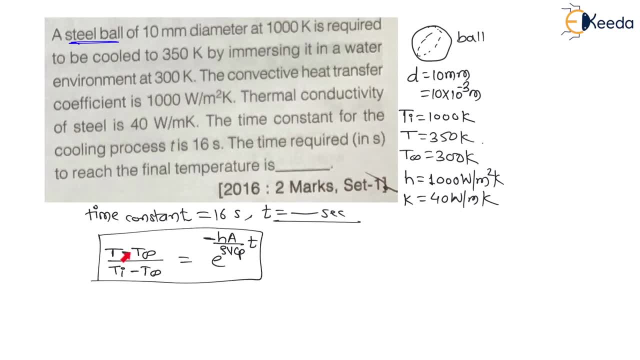 Right Now, my dear students, can I say this equation is a unitless Here: temperature divided by temperature, Kelvin divided by Kelvin, or degree Celsius divided by degree Celsius. It is a unitless or it is dimensionless. Right, It must be unitless. 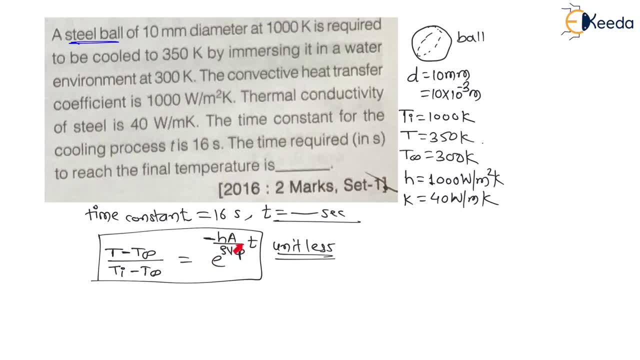 Therefore, this exponential to the power, this must be unitless Right. Therefore, my dear students here, This h a divided by rho v c, p into T, is unitless, is unitless Right. And we know that the unit of time is second. the unit of time is second. 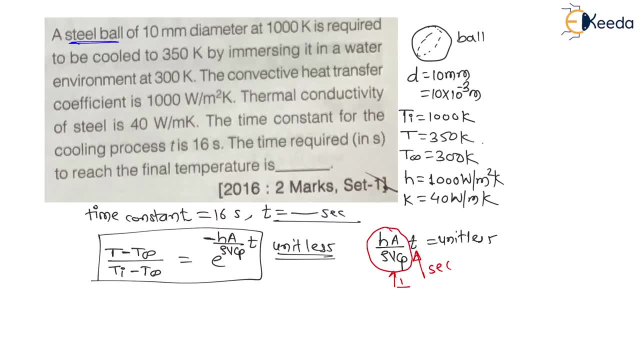 Therefore, this complete term must have unit of one upon second, one upon second rate. And, my dear students, the reciprocal of this, reciprocal of this is called time constant. Therefore, here the time constant, time constant which is nothing but in second, is nothing but rho v, c, p. 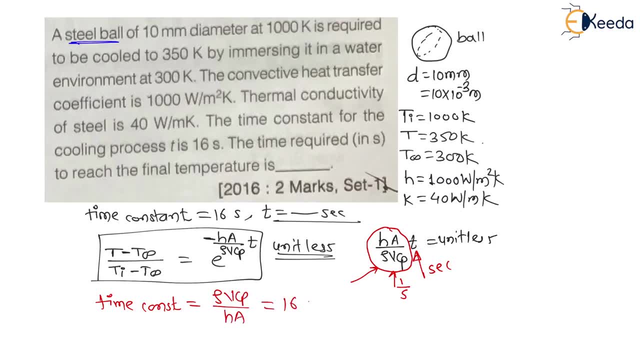 And this constant they have given 16 seconds. The reciprocal of this will become second as one upon second. the reciprocal of one upon second is second. Therefore, this value they have provided Therefore here, h, a divided by rho, v, c, p is nothing but one upon 16.. 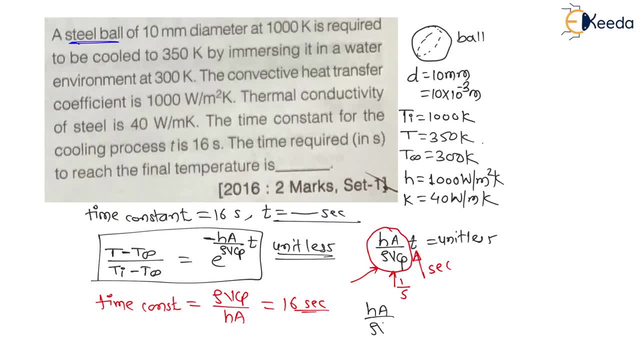 Therefore, can I say h? a divided by rho, v, c, p is equal to one upon 16.. Right, One upon second, one upon 16, that is one upon second unit Right. So, my dear students, this complete term, This is given, all the templates are given and our target is to find this time, 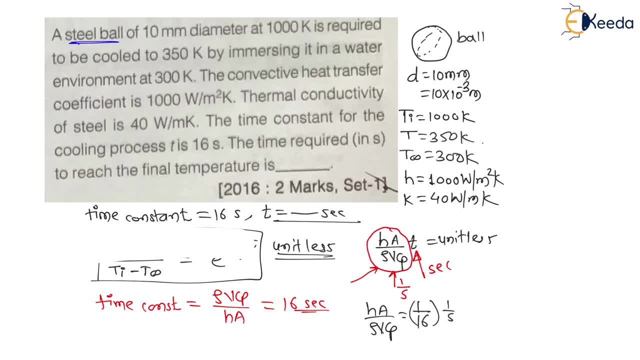 So let us use this formula and let us find this time Right. So, my dear students here, So we understood that what is the given term time constant is nothing but rho v, c, p divided by h, a. This is called time constant. Just now we have written.